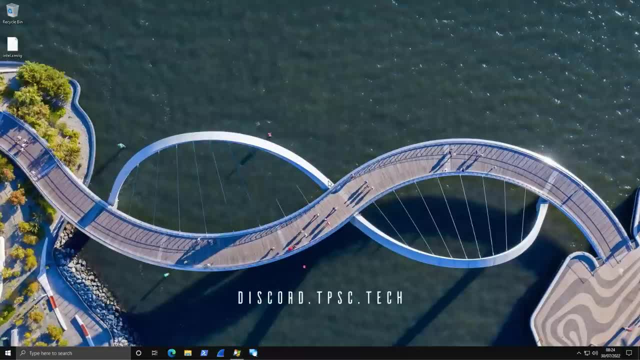 going to look at your system right after this video premieres, So make sure you go to discordtpsctech or follow the link in description for that. Now to kick things off and make this a really interesting video, we have a wonderful volunteer on the desktop. It's called intelxmrig. The second 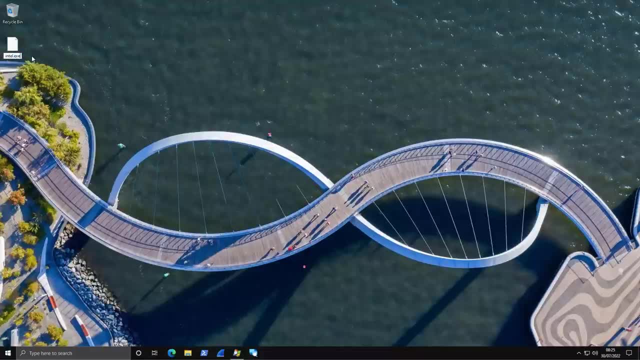 part of the extension might give you an idea about what it does, but we're going to go ahead and run it Now. some of you may think that anytime there is a malicious actor active on your computer, if you're hacked, you're going to have a malware process or you're going to have 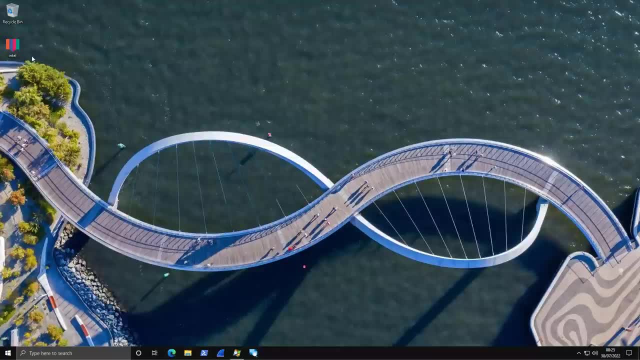 some sort of malware running that you can scan, that you can see in your process list, or you can upload to VirusTotal and check the detections of, or something an antivirus scanner is going to pick up. But, as we'll see here, that is not necessarily the case. So after running, 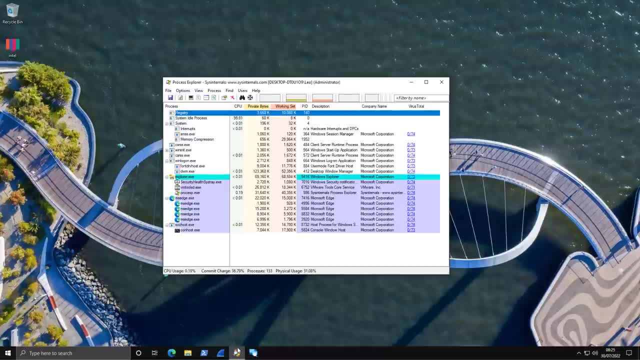 this sample. I'm just going to open up Process Explorer and, as you can see, we do not have a malicious system running on the system. It looks nice and clean and good to go, But as we'll dive deep, you will see that we have a crypto miner embedded within the system. that is going to be. 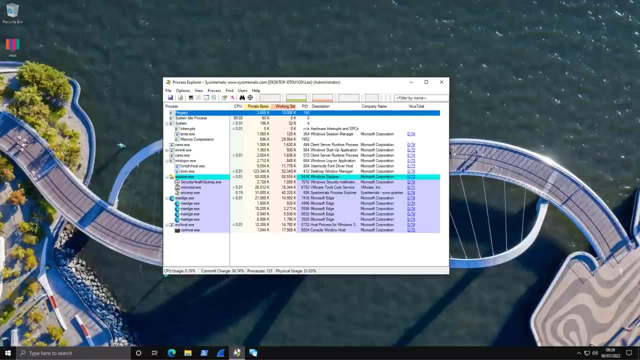 taking up CPU resources and profiting the attacker. Another thing to note before we get started is all the tools I'll be using in this video are basically part of the sysinternal suite, So there's no paid tools. These are all free that you can download directly from Microsoft. You can. 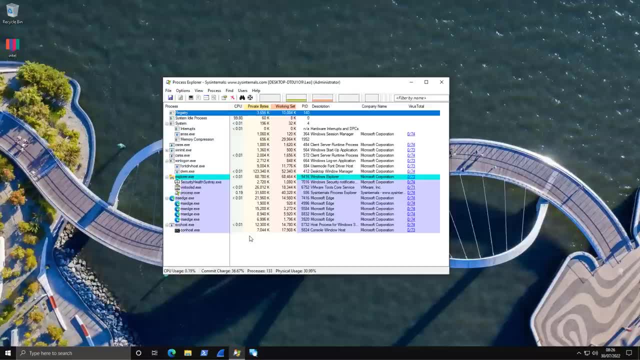 of course, dive into the sysinternal suite, and you can download the sysinternal suite from Microsoft Deeper with Wireshark- but we don't really need to do that, because what we're trying to establish is a connection to a certain malicious IP, And what we want to capture is the malware actor's. 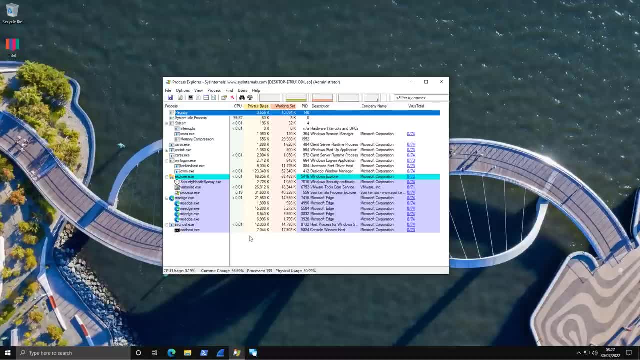 IP address, because that is going to allow us to not only shut down the malware activity on our system, but also report them to authorities to get them shut down in general. You don't necessarily need to actually look at the communications or the packets that are being. 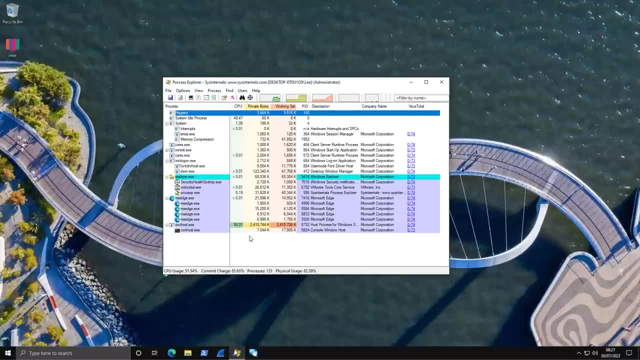 sent back and forth. What you really need to know is that you don't necessarily need to look at the communications or the packets that are being sent back and forth. You don't necessarily need to know is if there is a suspicious connection being made And as we're talking, you can notice. 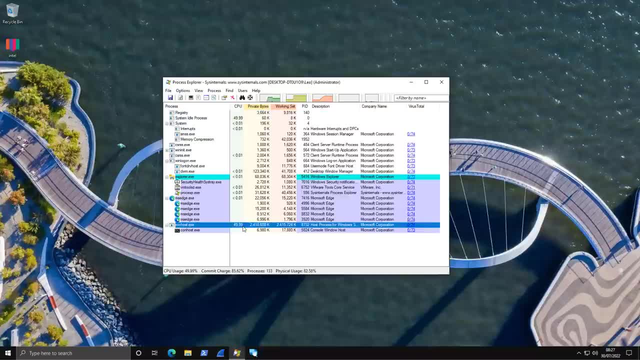 svchostexe all of a sudden starts to take up 50% of the CPU. Look at the RAM. It's taking up as well, And it says it's a host process for Windows system and it's correct. So what's happening? 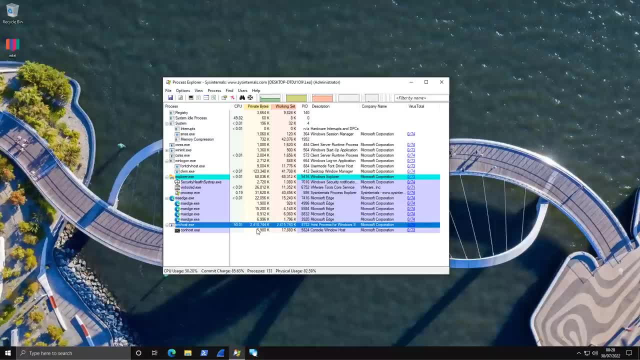 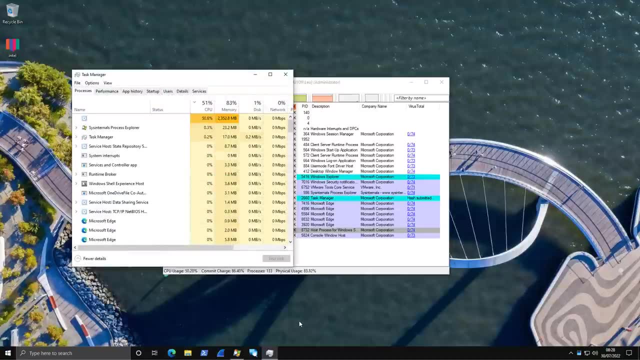 here Hard to tell unless we look at the network activity. I'm also going to open Task Manager just to show you what a typical user would see. So there's no malicious process here. We just have the system taking up 50% of CPU. If you're an average user, you might think that this is just. an update, especially now that updates do actually persistently cause annoyances such as this. But, as we'll discover when we check the IP address, this is not an update. This is a crypto miner mining Ethereum, likely on our system. So how are we going to do that? Well, first step. 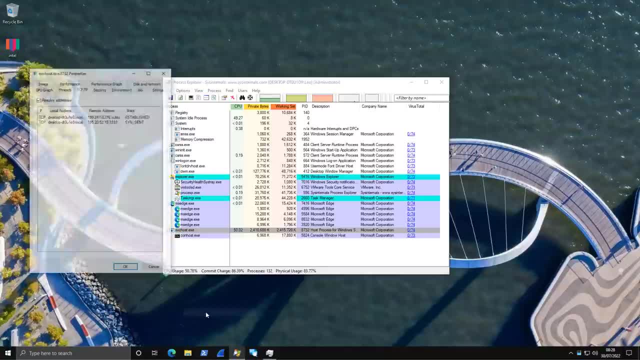 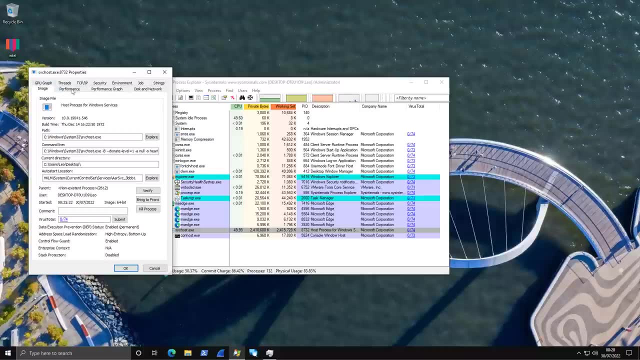 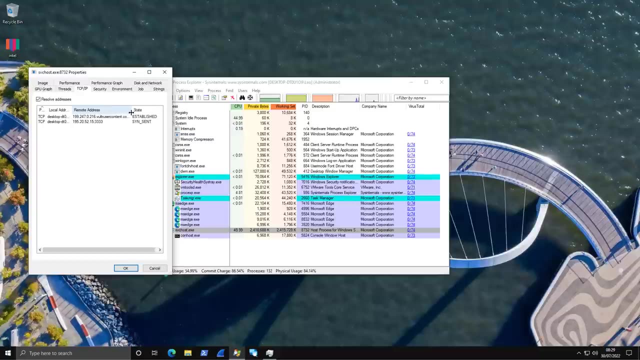 we're just going to right click on this and click on properties And within these sections, it's typically going to start at image. You need to go to TCP IP And this is going to show us the different network connections established by this particular 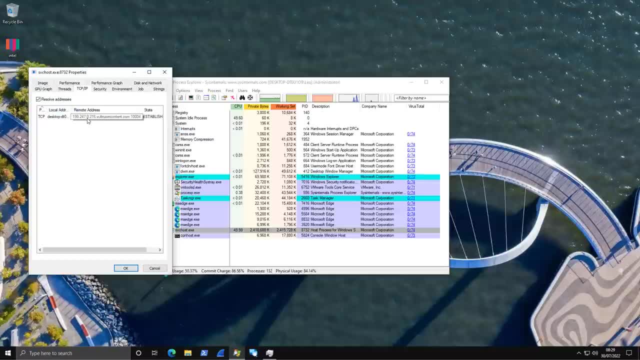 process. As you can see, we have a remote server here, We have two of them in fact- And these are likely nodes that the threat actor is using to run their malware operation. Sometimes these can be a third party, like they may be a Google server, an AWS server even, But if that's the case, what you 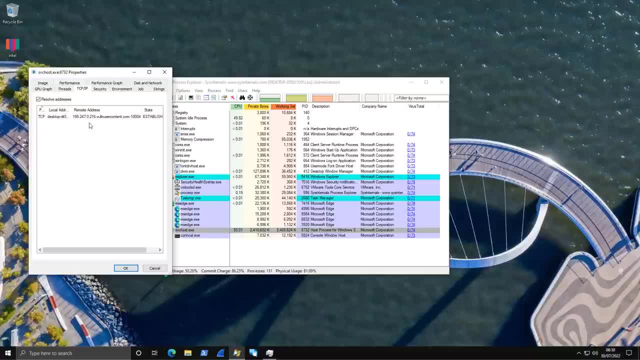 can do is you can collect this IP and write down a complaint saying that this particular IP address is being used for malicious purposes, And the vendor who's providing services to the threat actor should be able to shut them down, because that would be against their terms of service. 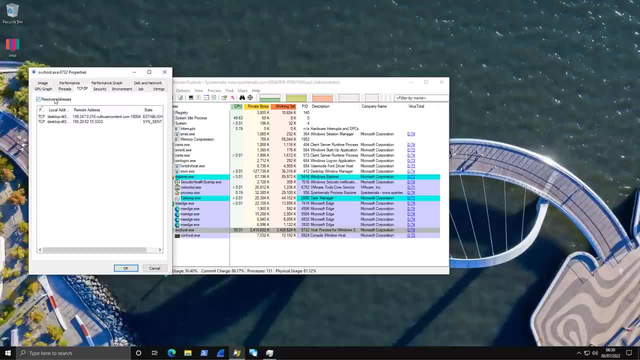 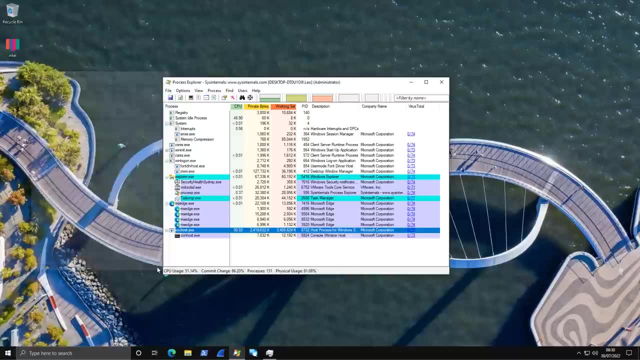 Make sure you have the resolve addresses checked over here, because that's going to show you more details. If we go back to the original IP address, we're going to see that the IP address is being sent to HTTP TCP, which is this IP address rather than the public address. When an IP address 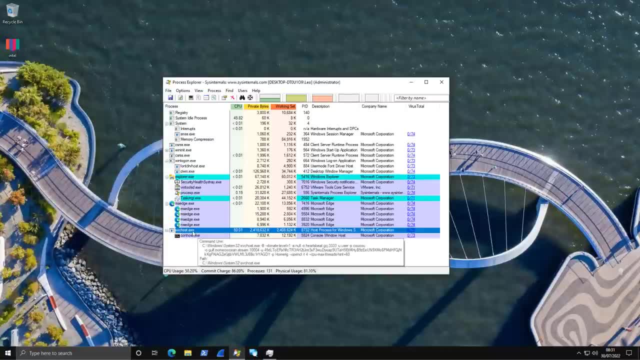 isices. we're just going to check it And we're going to see the IP address that's been sent to just this particular IP address. what's the data we're looking at? And in the starting source shell we just need to say: well, okay, So IP address is going to show up. what's the status? 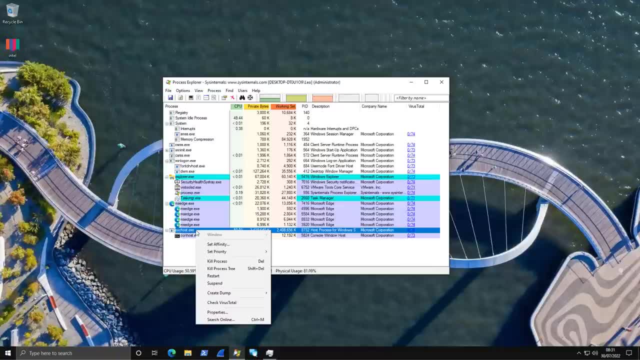 target and what things are we sending out there? So type p, caseific, different per language. We're going to have to give A if i'm using the organization with the conversationwise endpoint class key, but maybe we can outwit some orders to see what we 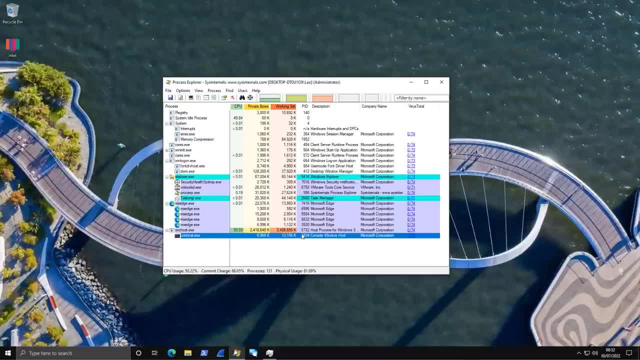 're getting into. So the IP address I'm pressing while we send thatей and I'm going to save the IP address to my user And this is what you're seeing. So what I'm seeing here in our away, what we would have to do is look for any persistence mechanisms that it may have on the. 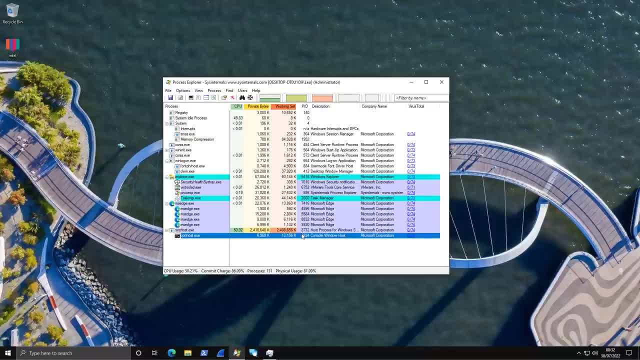 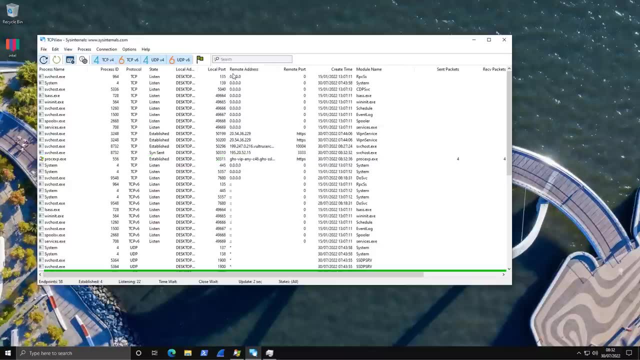 system, which is something we discussed in the last video, So if you haven't seen that, make sure you go and watch that one. To get a better view of this, though, and also to get a summary of all the connections your computer is currently making, you can go to TCP view, which is also a part of 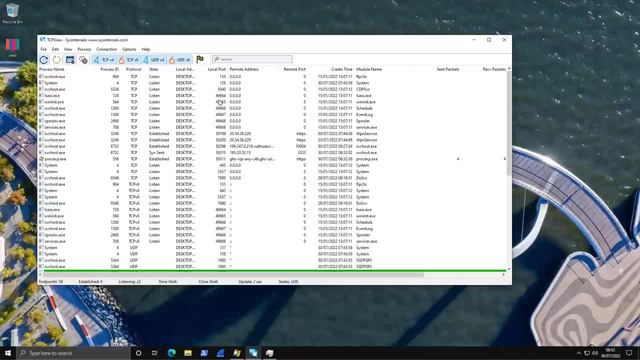 Sysinternals And this is going to show us all of our different processes and the remote addresses they are connecting to. Now you can see some of these are legitimate Windows services. Once again, make sure you have the resolve addresses checked over here. But this one is definitely suspicious. 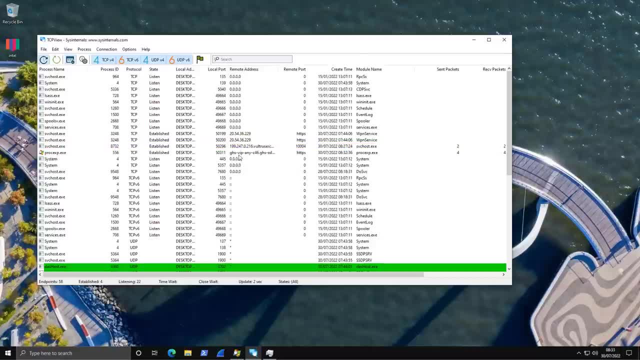 as is this one, because they are not standard IP addresses that I would normally see on a system. But, of course, if you're a new user, you may not know that. So how can you determine which of these are legitimate connections being made and which of these are suspicious? Well, for starters, 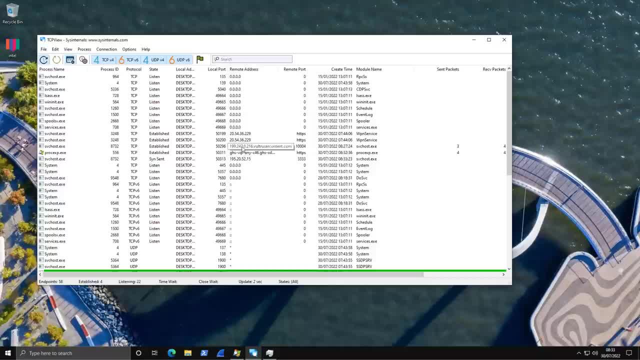 you can check if any network activity is supposed to be happening on your computer. So if you have, for example, Steam Discord and all of that running, you can try shutting down those applications. That's going to reduce some of the noise here And that way you're going to be able to isolate if there's anything happening beyond. 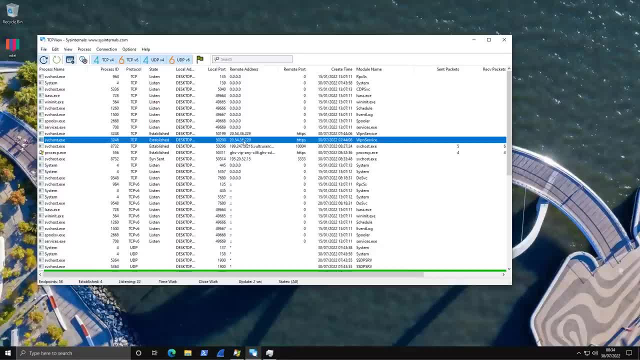 what you expect. Once you've done that, what you can do is you can obviously copy the particular IP address and then look it up and see if it is associated with a legitimate service, Or you can just right click over here and click on who is, and this is going to get. 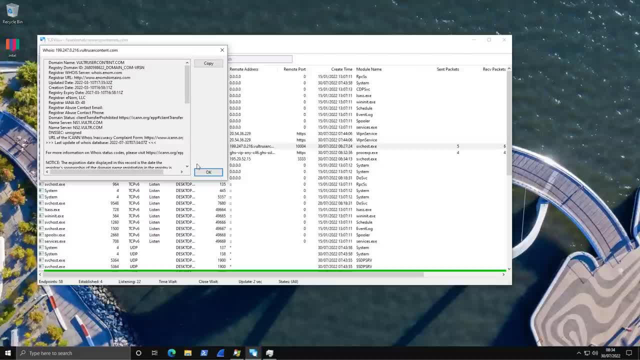 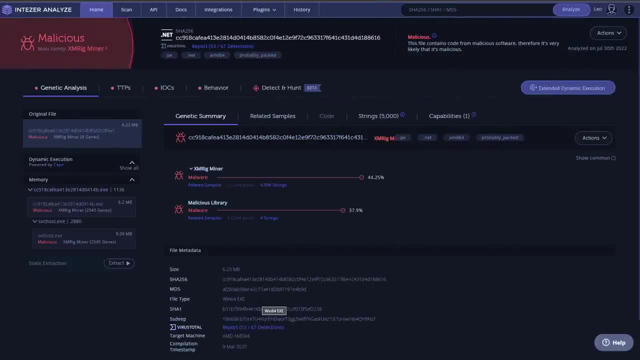 the details for the domain name and who it's registered to. You can also get a complaint form here and report the threat actors And, of course, once you have isolated the original sample, you can analyze it on a web platform like Intazer or Varstotal. A big thank you to our sponsors. 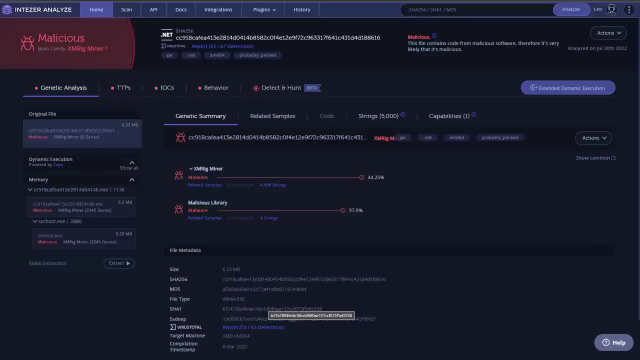 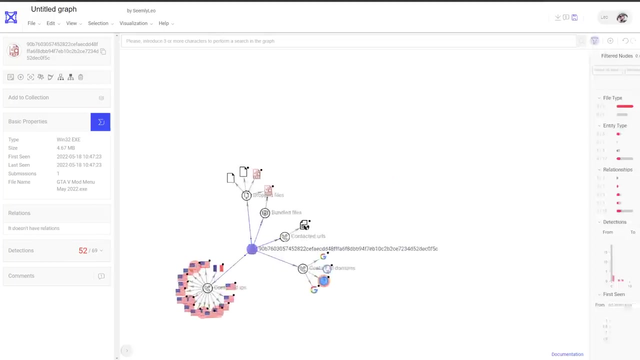 Intazer for setting up an enterprise account so we can do our threat investigations. So, as you can see, this particular threat is an XMRigMiner. It's got a 44% correlation with that. We check the report. We've got 53 detections. But once again, a reminder that this is not the first thing you 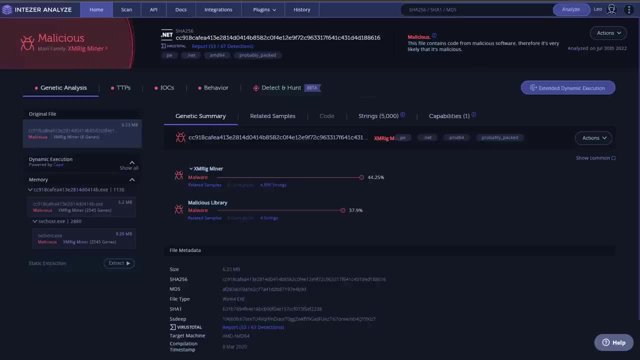 might see when you look at a compromised system. So you may have a system with only legitimate looking processes. that is totally malicious And, by the way, these crypto miners are very clever. So what they might do is, when you open up something like Task Manager, they just drop all of their. 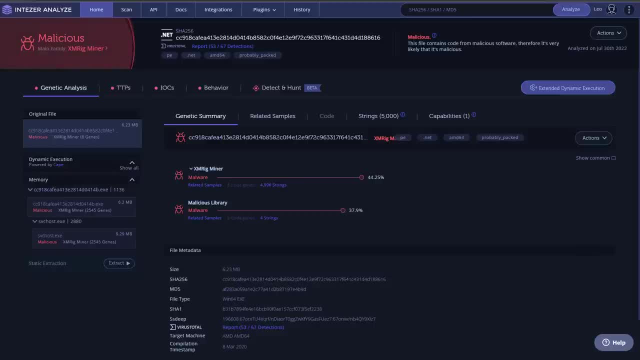 resource usage. so you don't see anything strange. But when you go away, in the background the miner starts ramping up and taking up all of those CPU resources. Now if we look at the dynamic execution in the sandbox here, you can see that in memory it has the same behavior that we noticed. 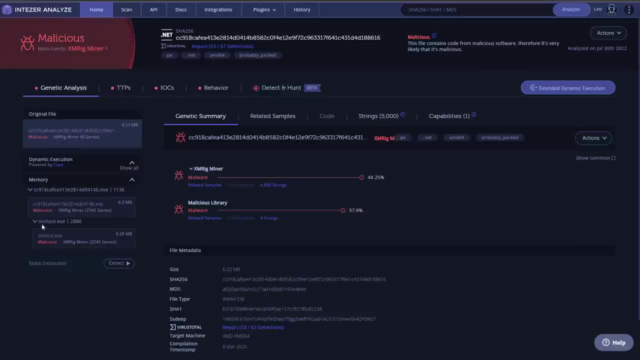 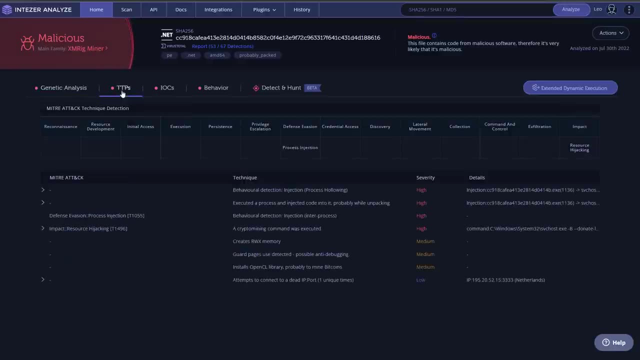 in the virtual machine. So it launches svchostexe, which looks legitimate, but is what carries out its mining operations? We take a look at TTPs. We've got process injection here, use of process hollowing. This is a technique where attackers basically replace a legitimate 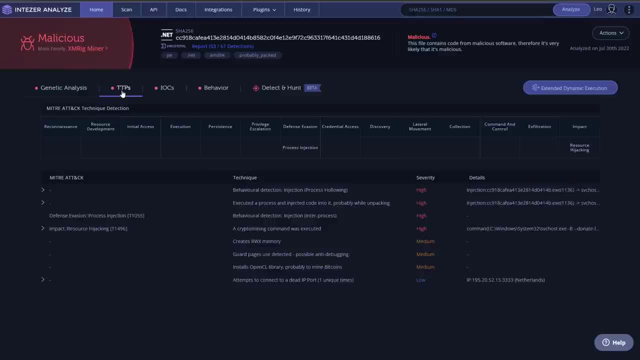 system process. They use it for their malicious activities. We've also got a crypto mining command, which is what we also saw on the system when we're looking at Process Explorer. It's basically the same string and instruction set And we've also got this IP. This one leads. 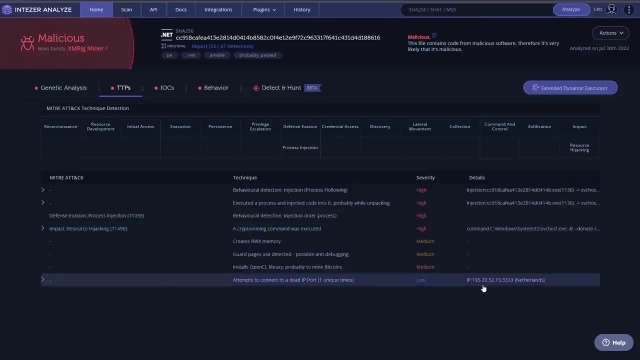 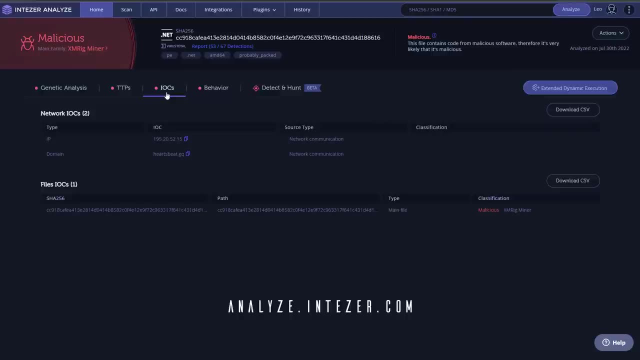 to the Netherlands. By the way, if you would like to conduct a similar threat investigation, you can set up a community account on analyzeintrudercom and start using it for free using the link in the description. Now back on our screen. 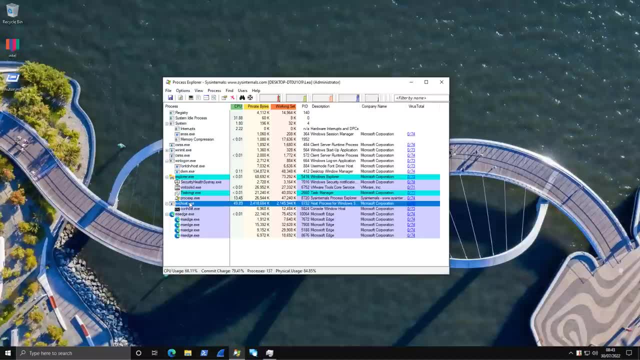 In our system, we can go ahead and terminate the process tree that is associated with the crypto miners. I don't want to keep making them more money, But hopefully that demonstrates how malicious network activity can be spotted on your system. So once again, going through the steps. 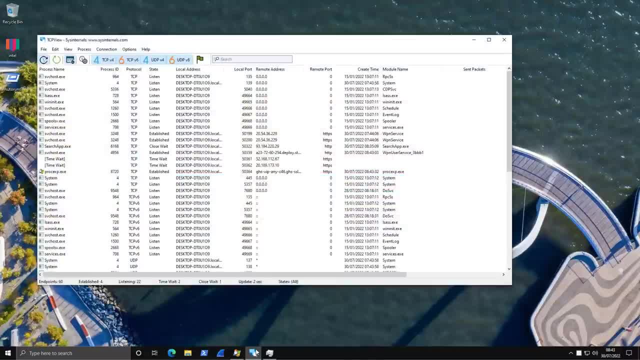 you want to open up something like TCP view, look at the remote addresses your system is connecting to and then try to resolve them and see if any of them don't add up or are not connected, And then, once you're done, you will see a demarcation of your system within a second. 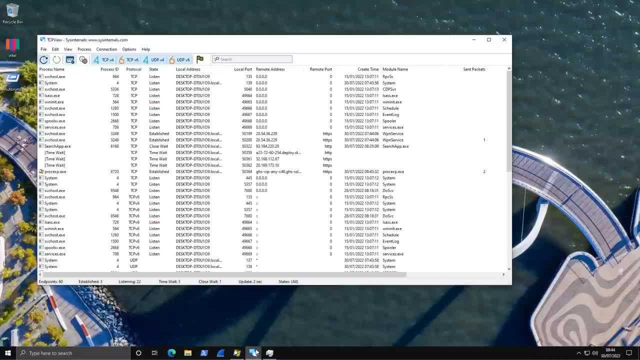 In the future, we're going to focus on more in-depth analysis of different aspects of malware, So don't forget to subscribe to the PCSecurity channel if you'd like to learn more about cybersecurity. Now we're going to be doing a live analysis of. 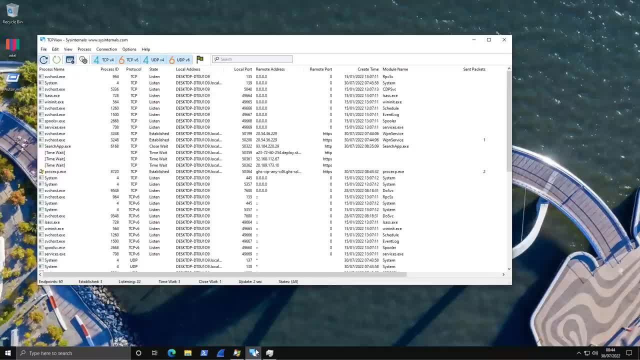 whatever's happening on your system in our Discord workshops. So click the link in the description, go to discordtpsctech to join our event and I'll be there to help you practice some of the concepts discussed in this video and walk you through the process of conducting a threat investigation. So 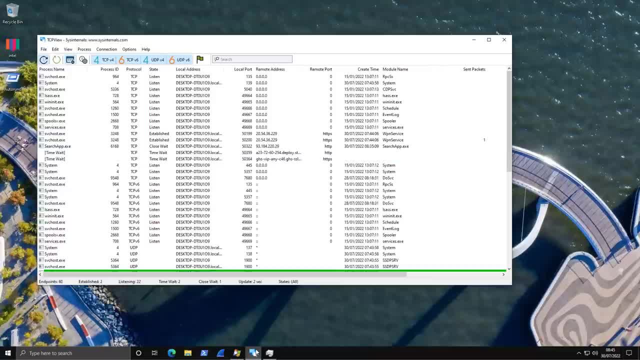 if you have any questions, that'd be a great place for you to ask, because I will be there live with our awesome community. So don't miss out on the event. It's a great chance to meet some amazing people, So I will see you there at discordtpsctech. I hope you found this video helpful. 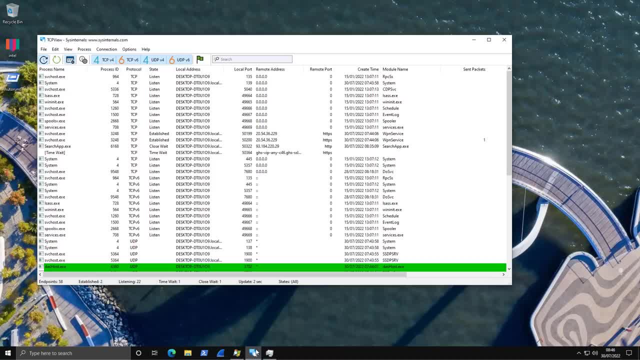 Please like and share it if you'd like to see more such content in the future. This is Leo. Thank you so much for watching and, as always, stay informed, stay secure. 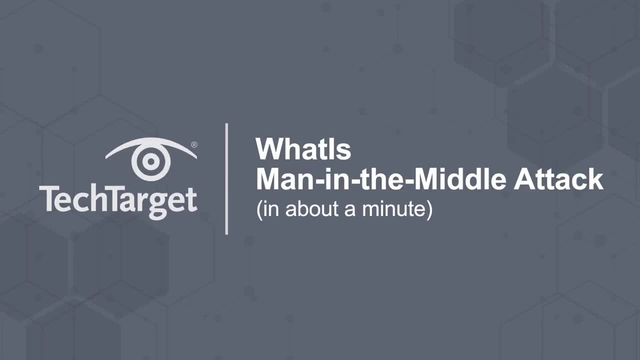 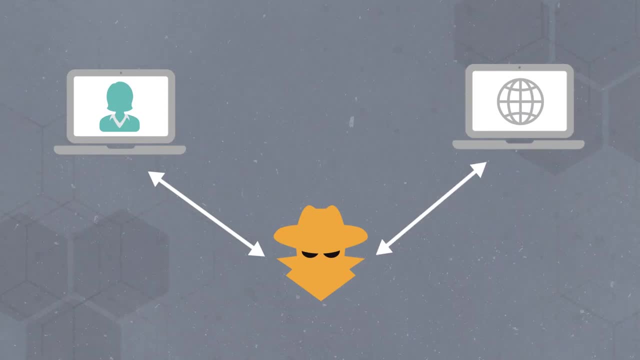 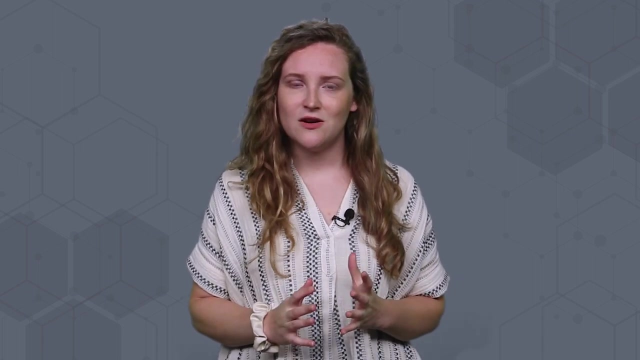 A man-in-the-middle attack is a type of cyber attack in which an attacker intercepts and relays messages between two parties who believe they're communicating with each other. Man-in-the-middle attacks pose a serious threat to online security because the attacker can capture and manipulate. 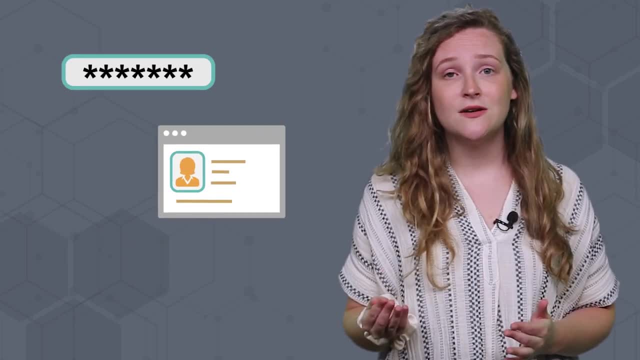 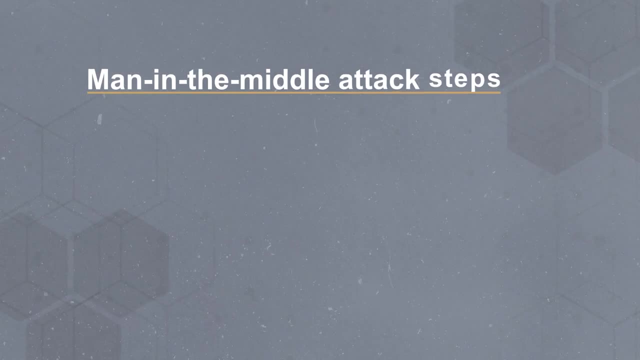 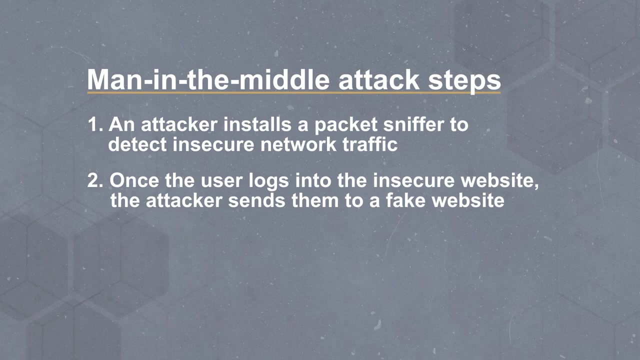 sensitive data like login credentials, account details or credit card numbers in real time. Man-in-the-middle attacks typically follow these steps. An attacker installs a packet sniffer to detect insecure network traffic. Once a user logs into the insecure website, the attacker sends them to a fake website. The fake website mimics the original website. 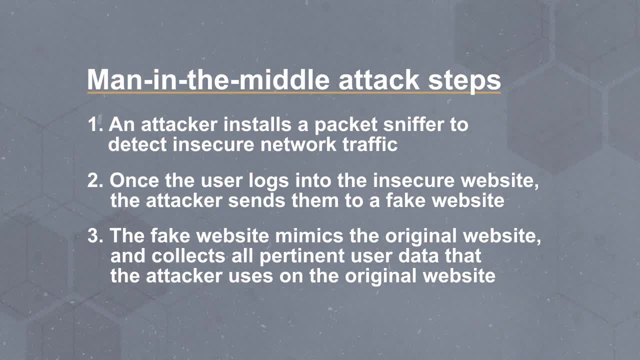 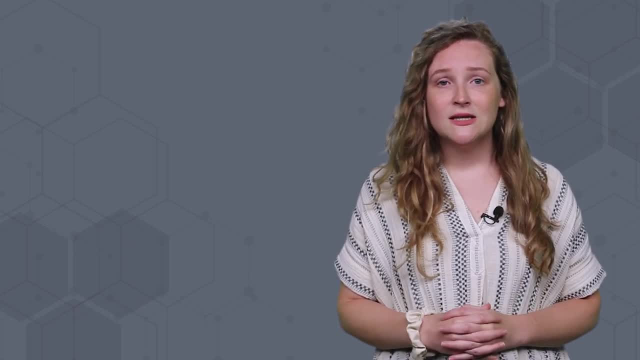 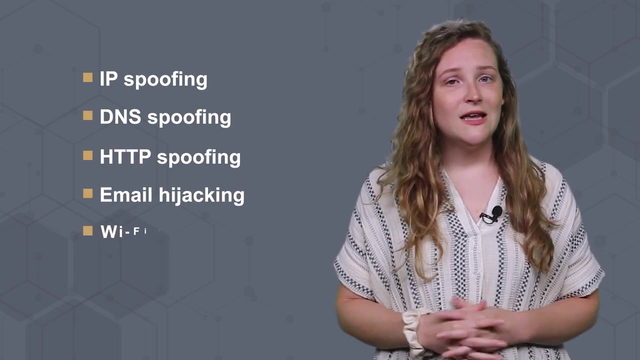 and collects all pertinent user data that the attacker then uses on the original website. Cyber criminals conduct man-in-the-middle attacks in a variety of ways, including IP spoofing, DNS spoofing, HTTP spoofing, email hijacking, Wi-Fi eavesdropping and cache poisoning, among others.